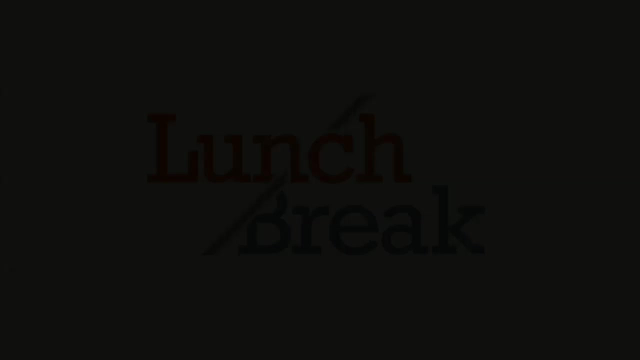 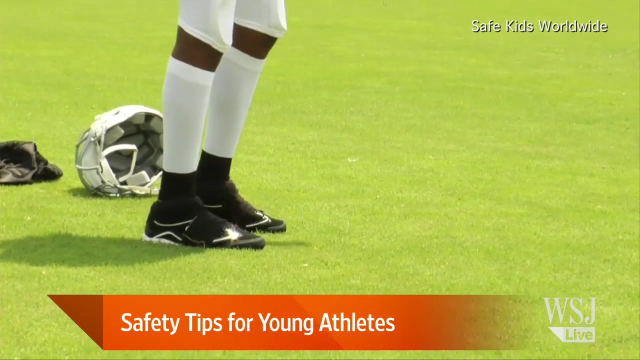 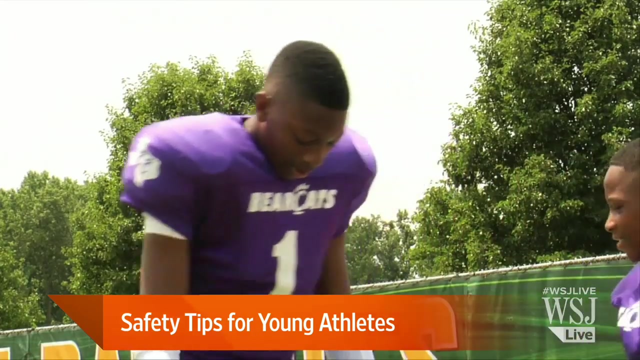 Every day, over 3,000 children sustain a sports injury severe enough to go to the emergency room, and the greatest number of injuries are in kids just 13,, 14, and 15 years old. To better understand what's happening here, Safe Kids Worldwide conducted a survey of parents, coaches and young athletes. 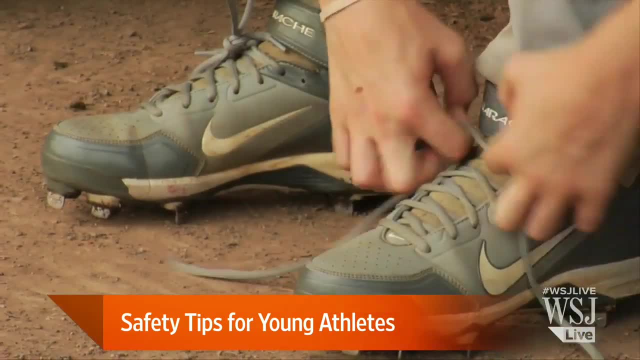 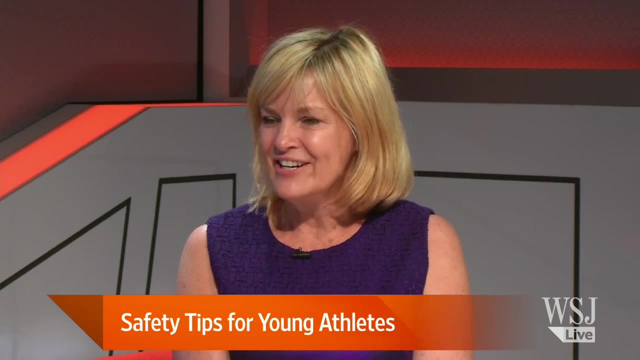 to explore how the culture of sports may be. what's keeping kids out of the game? Here to tell us more is Kate Carr, president and CEO of Safe Kids. Kate, thanks so much for being with us. Oh, thanks for having me. These are really scary numbers, these numbers of injuries in kids so young, and it seems to be on the rise. Well, when you look at the total number of injuries, it's about 1.24 million in 2013.. That's emergency room visits alone. 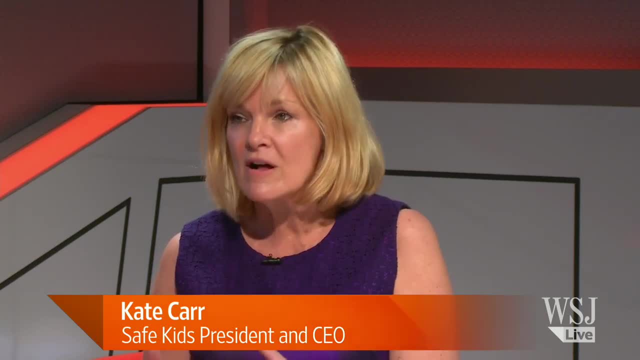 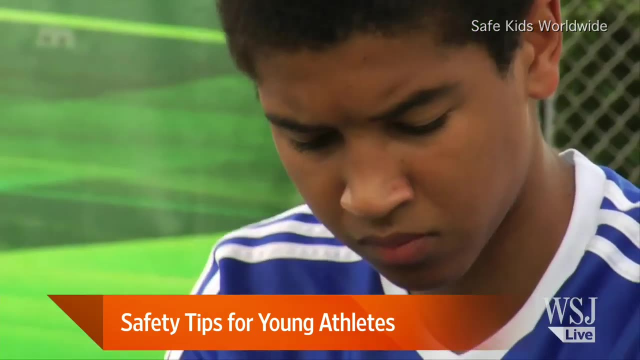 And if you think about the cost of that to families, that's close to a billion dollars in health care costs. So are we looking at a greater increase? We're seeing a large number of kids and no matter what the number is, it's still way too many kids. 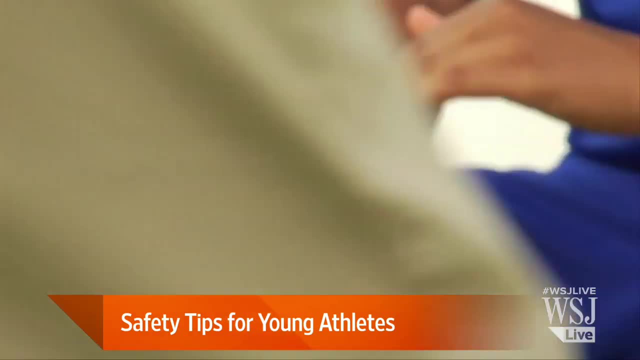 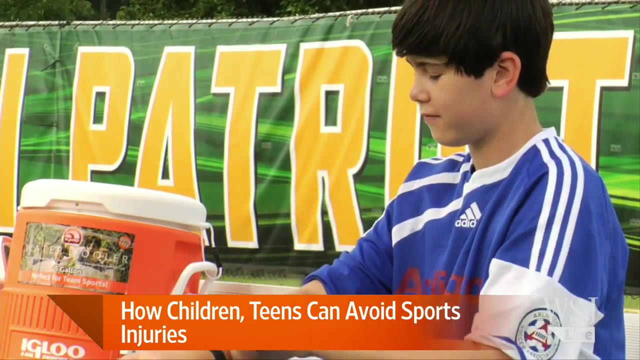 Way too high, absolutely. So what's the role that parents are playing here? I mean they should be protecting their kids, but are they sometimes making this worse? Well, parents told us that they felt that coaches had the training that they needed, not only in the sport, but in injury prevention. 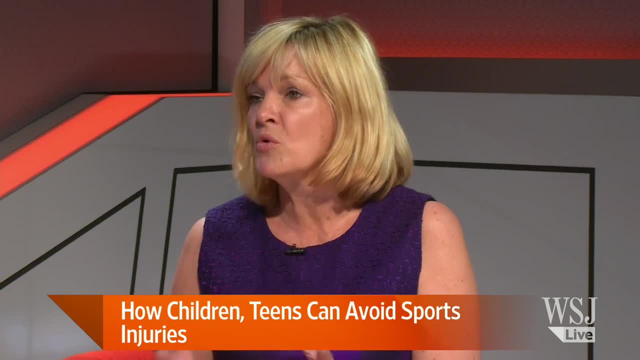 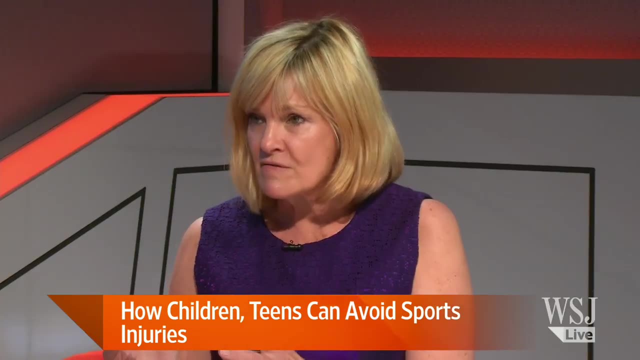 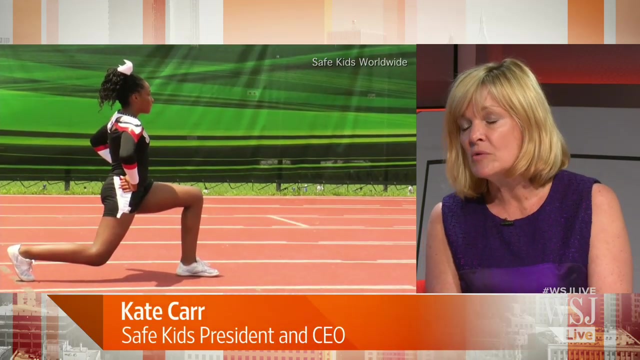 Yet coaches told us more than 50% of them wanted more training in injury prevention, So they don't have the training necessary for the most part. Well, there is. There are specific areas of training so you can have concussion training, AED, CPR, but overall injury prevention. that training doesn't exist now and we'd like to see that developed and happening. 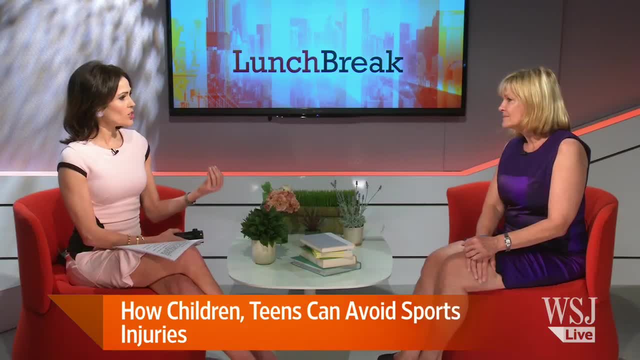 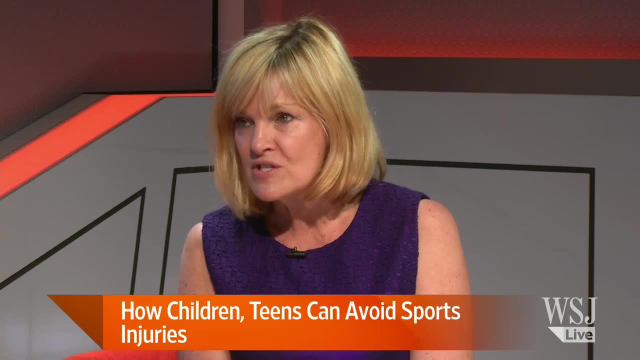 And as the pressure to perform intensifies, are coaches pushing the kids harder. Well, coaches could be pushing the kids, but we also found that parents were pushing coaches to play kids, even when kids were injured. And what were kids telling you? 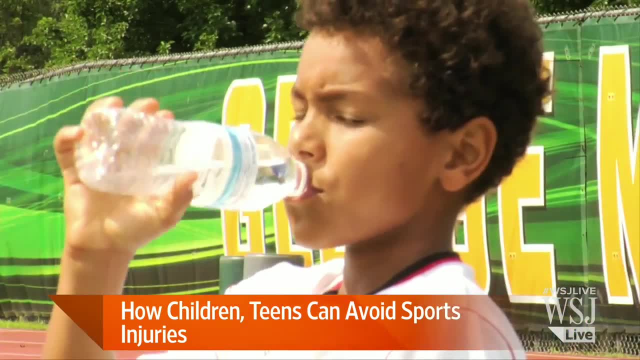 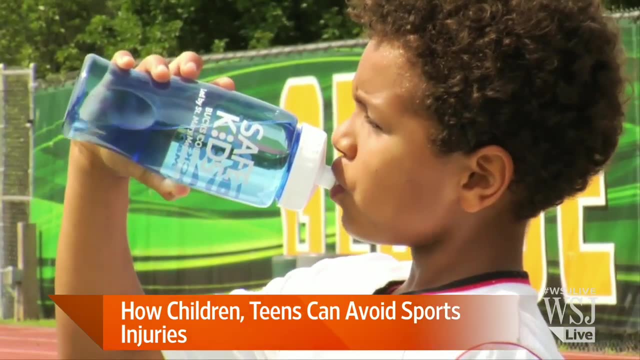 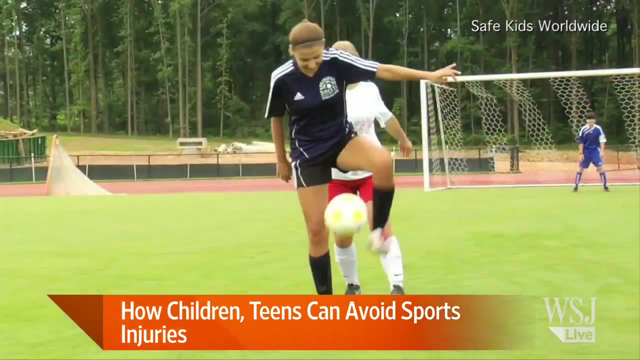 I found it so interesting to hear what kids playing injured would say about it. Well, 42% of the kids that we interviewed said that they had played injured at some point in time. But even more alarming was, one of every four kids told us that it was okay for them to have a hard hit, a late foul, something that you could call dirty play. 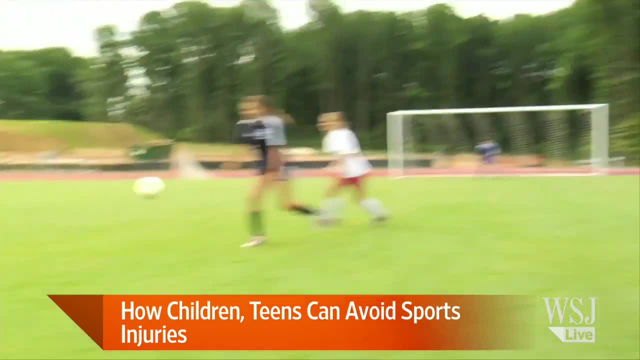 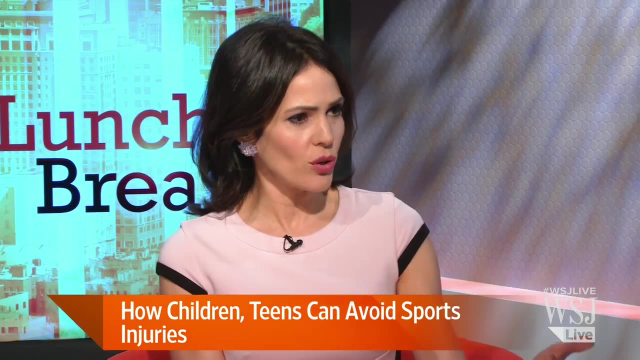 Absolutely Something that just didn't belong in the game, And a lot of them were getting injured- 33% of them were getting injured as a result of dirty play. So how can all groups involved- the children, the parents and the coaches- how can they stop this?